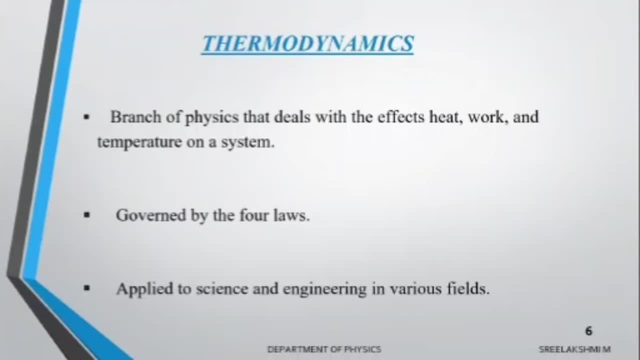 Thermodynamics deals only with large-scale response of a system which we can observe and measure in experiments. The small-scale gas interactions are described by the kinetic theory of gases. The methods complement each other. Some principles are more easily understood in terms of thermodynamics and some principles are explained by the kinetic theory. 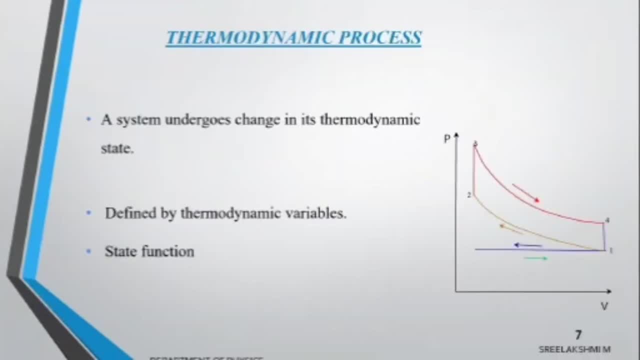 Thermodynamic Process. Now, how does the food stay cold and fresh in refrigerator? but have you noticed, even though the entire inner compartment of a refrigerator is cold outside, or the back side of the refrigerator is warm, in fact hot Here, the refrigerator pulls heat from its inner compartment and transfers it to the region outside. 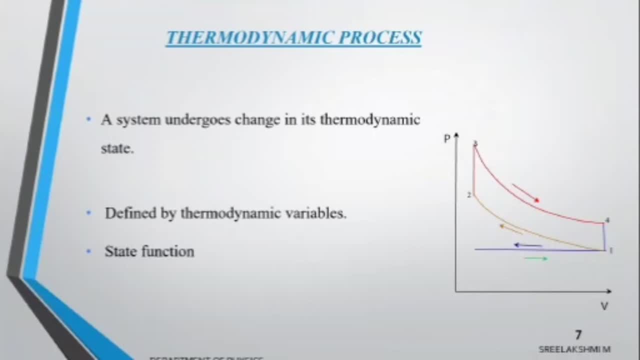 This is why the back of the refrigerator is warm to touch. So thermodynamic processes involve heat energy moving within a system or between systems. Now thermodynamic process is defined by change in the system. It is a passage of a thermodynamic system from an initial to a final state of thermodynamic equilibrium. 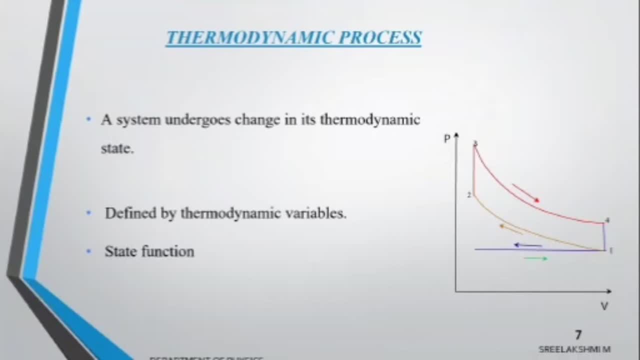 Now, the initial and the final states are the defining elements of the process. But the actual cause of the process is not of primary concern. And it is not of primary concern, It is often ignored. So a state of thermodynamic equilibrium endures unchangingly unless it is interrupted by a thermodynamic operation that initiates a thermodynamic process. 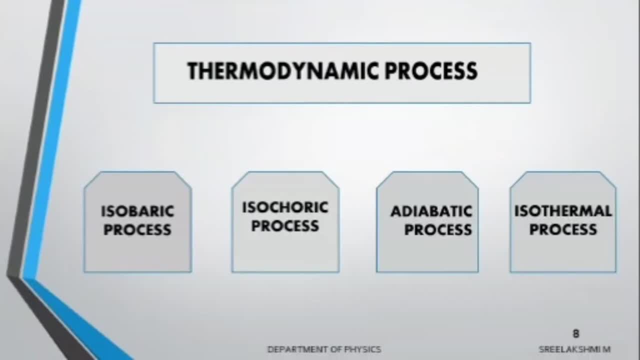 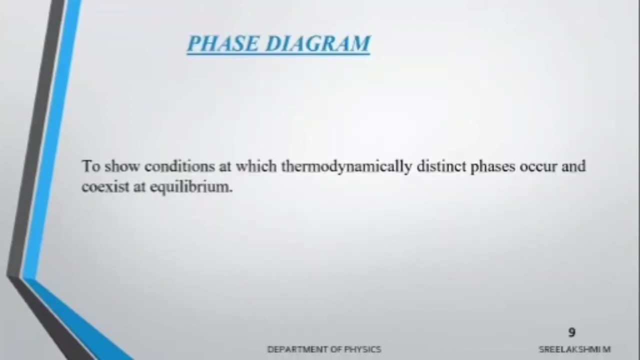 So today we will be dealing with four major processes and its applications: Isobaric process, adiabatic process, isochoric process and isothermal process. Phase Diagram- A phase diagram in physical chemistry, engineering, mineralogy or whatever science. 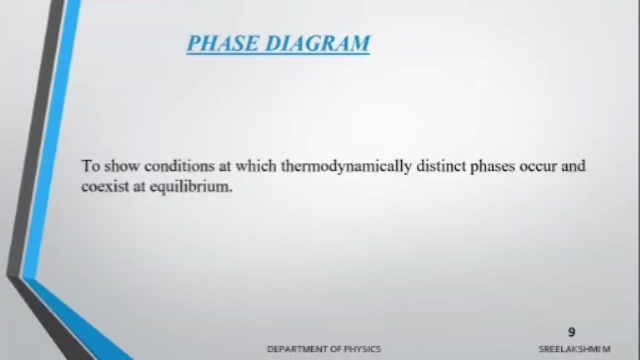 It is a type of chart which is used to show conditions like pressure, temperature, volume, etc. which are thermodynamically distinct phases, which they occur and coexist at equilibrium. There are two major kinds of phase diagrams: A two-dimensional diagram, which is pressure versus temperature. 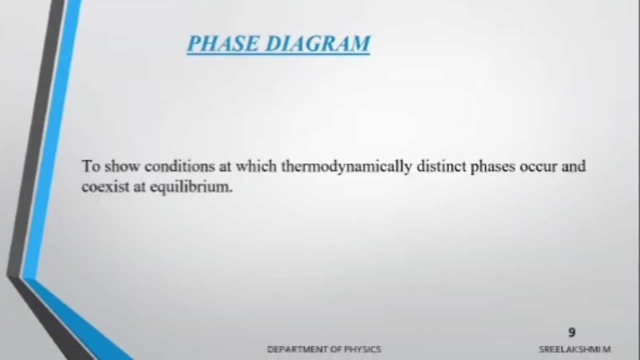 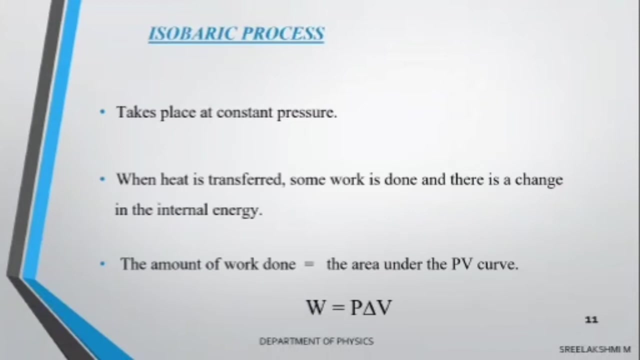 And the other one is a three-dimensional Which consists of pressure, temperature or volume, or any three together: Isobaric process. Now, what is isobaric process? An isobaric process is a thermodynamic process taking place at constant pressure. 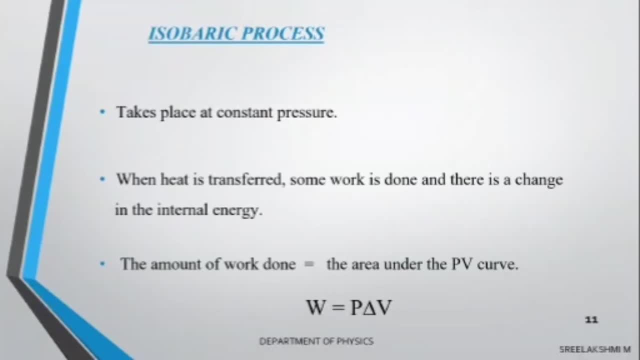 Like the term isobaric the word, it has been derived from the Greek words iso and baric, which means constant pressure. As such, the constant pressure is obtained when the volume is expanded or contracted, So which basically neutralizes any pressure change due to the transfer of heat. 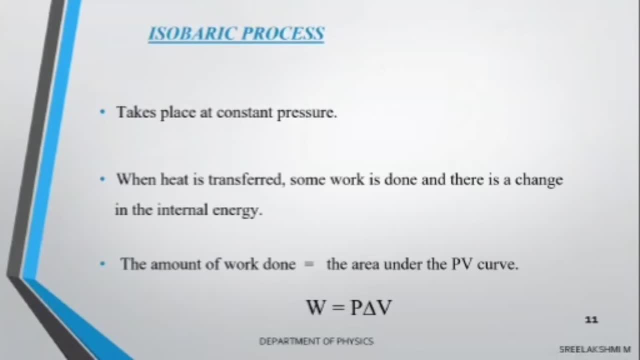 Now in an isobaric process, when the heat is transferred to the system. there has to be some work done So, however, even though there is no change in the internal energy of the system, this further means that no quantities, as in the first law of thermodynamics, becomes zero. 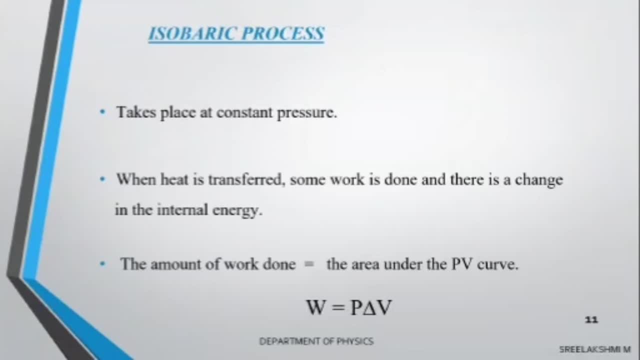 So the work done in a thermodynamic isobaric process is given by the equation. W, which is: the work done is equal to P delta V, where P is the pressure which is constant, and V delta V is the change in the volume. This is the PV diagram for an isobaric process. 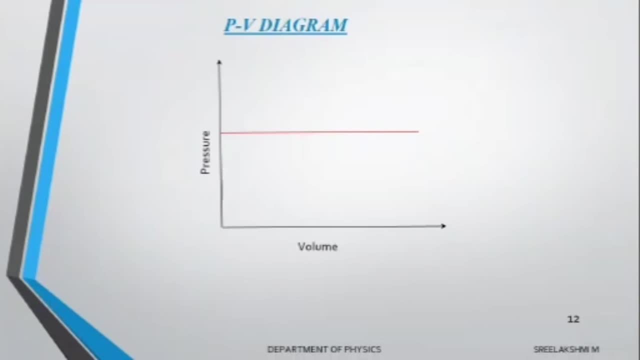 The work done by the gas is represented on the PV diagram by the rectangular area under the isobaric path on the diagram. Now, whether the area is positive or negative is dependent on whether the gas has expanded or compressed. The two applications of an isobaric process that I have mentioned here are: 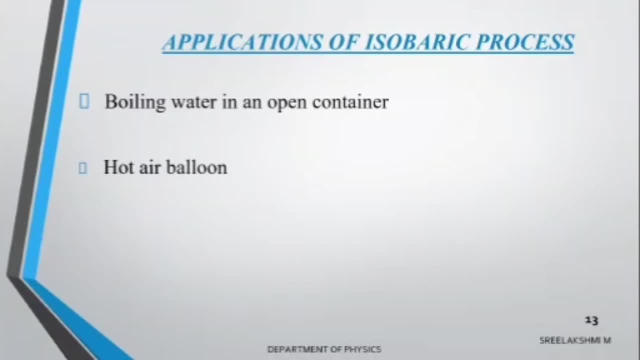 boiling of a water and hot air balloon. Now, boiling of a water is a very simple isobaric process. So you have a pot of water on the stove and it is at atmospheric pressure. Now, as the water boils, the steam coming off expands to roughly about 60 degrees. 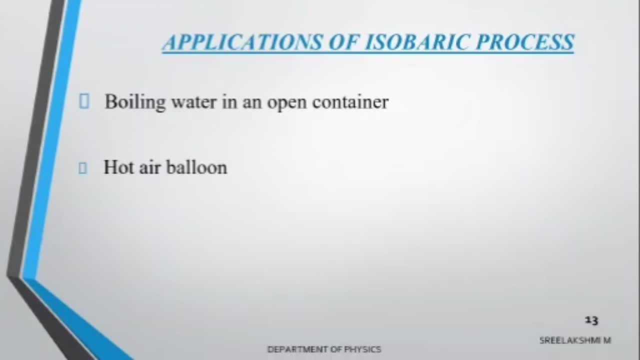 The steam comes off roughly about 1600 times of that of the water, And there is nothing to contain this steam, so it stays at atmospheric pressure. The next one is hot air balloon. A hot air balloon is lighter than aircraft consisting of a bag called an envelope. 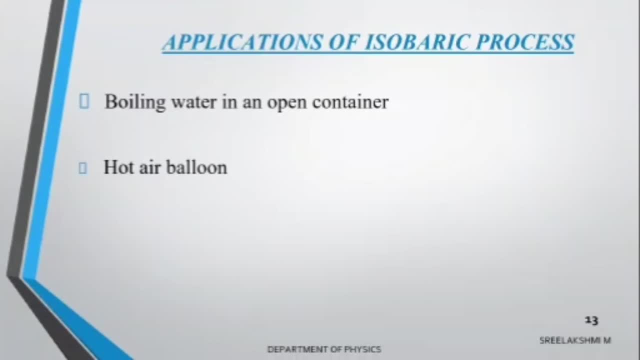 which contains heated air. Now, this heated air inside the envelope makes it buoyant, since it has a lower density than the colder air outside the envelope. As with all aircrafts, hot air balloons cannot fly beyond the atmosphere. The next process is adiabatic process, which will be dealt by Gopika. 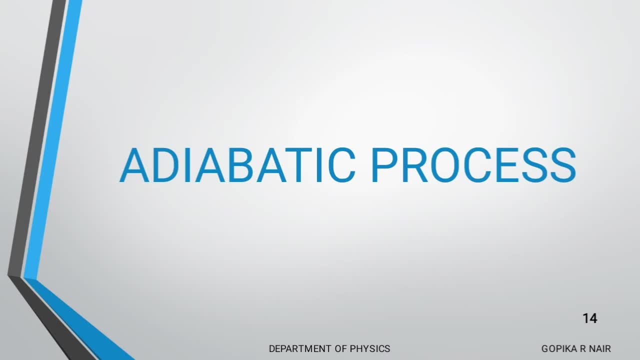 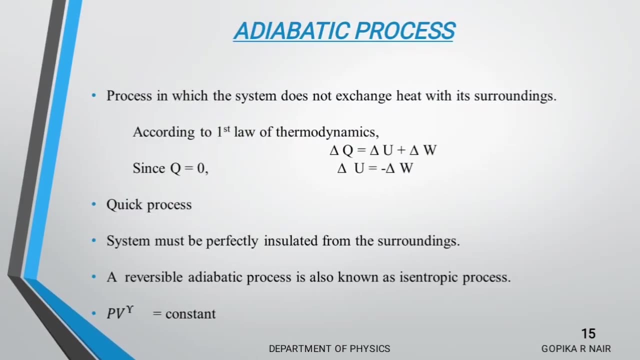 Now we are going to discuss another important thermodynamic process: adiabatic process. Adiabatic process is the process in which the system does not exchange heat with its surroundings. There is no heat flows in or out of the system. 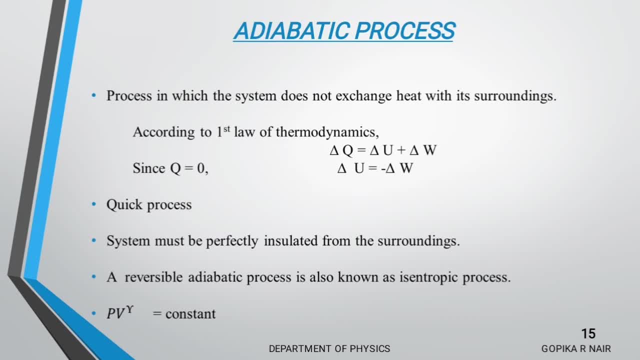 So the equation for first law of thermodynamics is: if the thermodynamics delta Q is equal to delta U plus delta W, here becomes delta U is equal to minus delta W. From this equation it is clear that if work is done by the system, 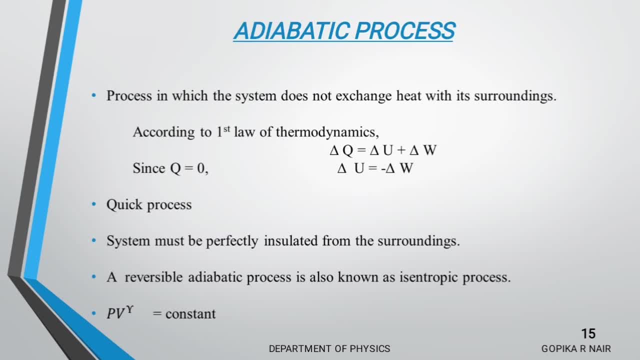 the internal energy of the system decreases by the amount of work, And also, if work is done on the system, the internal energy of the system increases by that amount. An adiabatic process is a quick process, So that there is no time to transfer heat. 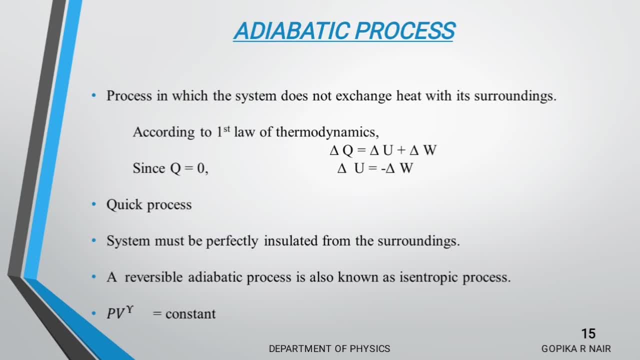 In an adiabatic process system must be perfectly insulated from the surroundings So that there is no transfer of energy, as heat occurs, between the system and its environment. A reversible adiabatic process is also known as isentropic process. 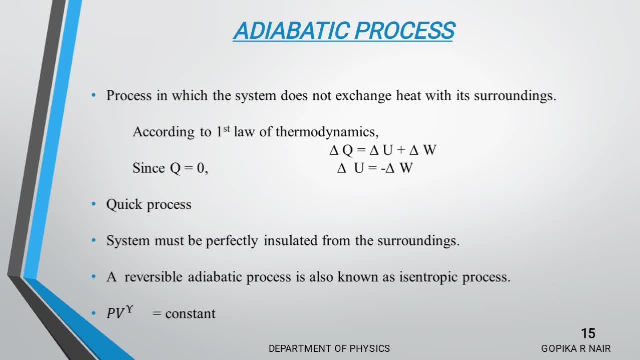 Because there is no entropy change, since there is no heat transmission. Following is the equation: for an adiabatic process, PV raised to gamma is equal to constant, Where P is the pressure of the system, V is the volume of the system and gamma is the adiabatic index. 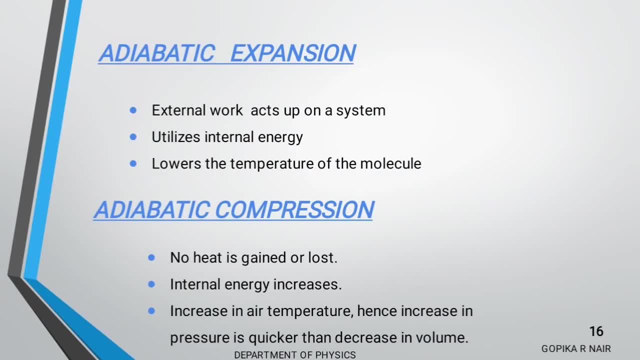 What is an adiabatic expansion and what is adiabatic compression? Adiabatic expansion is a situation whereby an external works acts upon a system at the expense of utilizing internal energy of the gas and results in lowering the temperature of the molecule of gas. 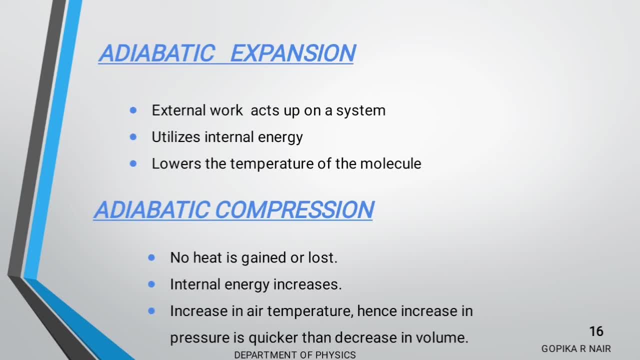 Adiabatic compression is a process in which no heat is gained or lost from the air And the internal energy of the air is increased. In this process, pressure increases quicker than volume diminishes due to increase in air temperature Work done during an adiabatic change. 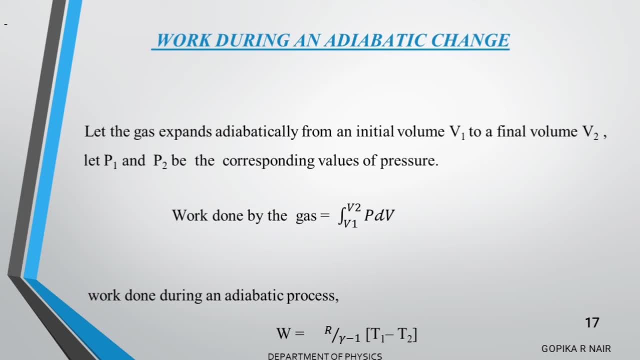 Let the gas expands adiabatically from an initial volume V1 to final volume V2.. And the corresponding values of pressures are P1 and P2.. Work done by the gas: integral V1 to V2 PdV. By integrating this value we get final equation for work done. 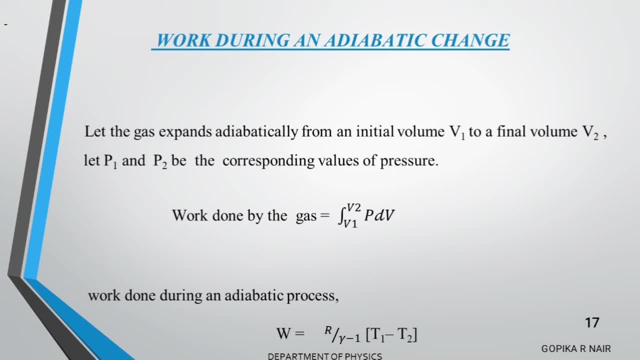 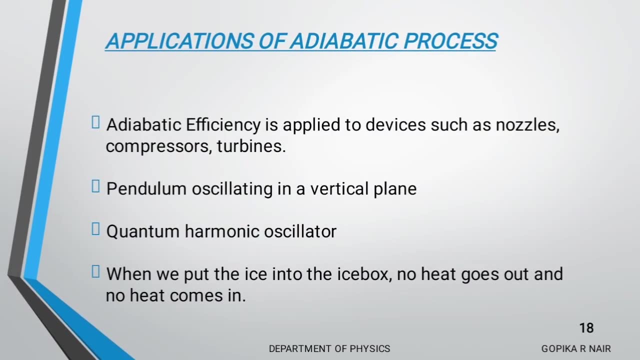 Work done during an adiabatic process is equal to R by gamma minus 1, T1 minus T2.. There are many applications for an adiabatic process. Some are noted below. Adiabatic efficiency is applied to devices such as no-sills companies. 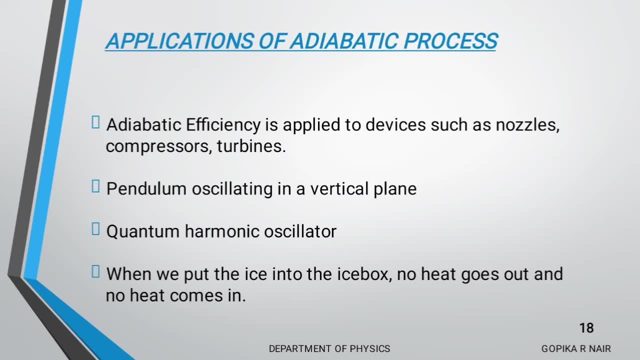 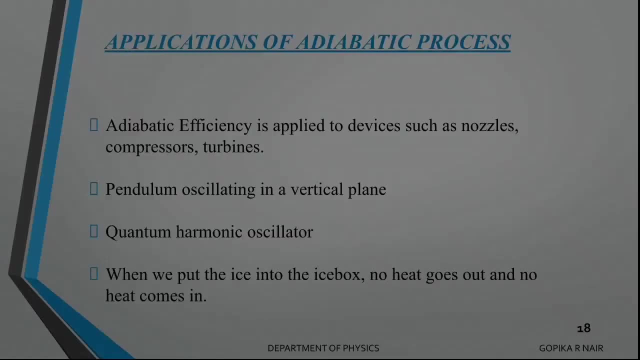 Compressors, turbines, Pendulum oscillating in a vertical plane, Quantum harmonic oscillator. When we put the ice into the ice box, no heat goes out and no heat comes in. These are some of the applications. Thank you, Hello friends. 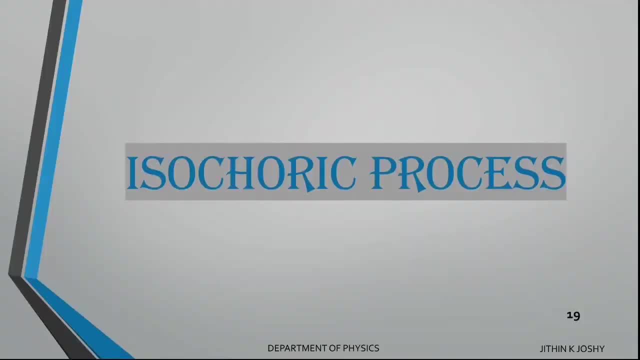 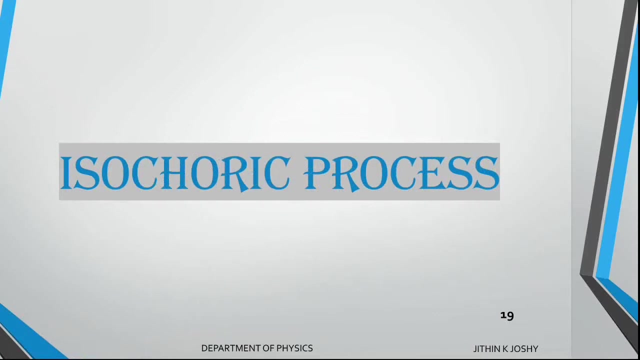 Myself, Jithin Kejoshi. So far, we have discussed about the various thermodynamic processes, such as isobaric process and adiabatic process. Now we are going to deal with isochoric process. An isochoric process is a thermodynamic process taking place at constant volume. 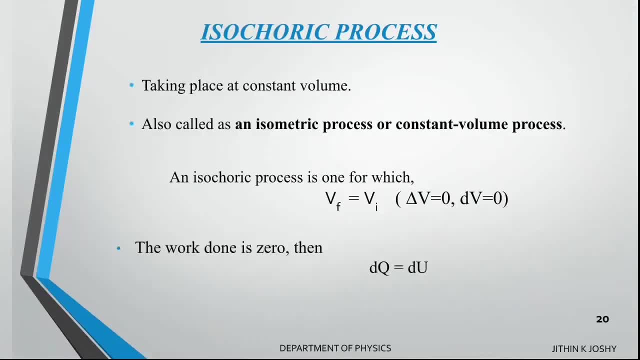 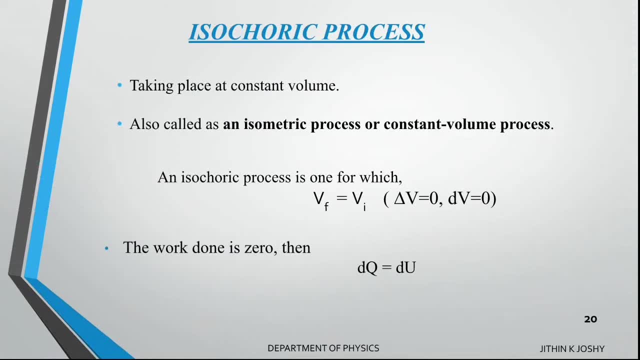 This process is also called as an isometric process or constant volume process. In an isochoric process, the final volume and the initial volume are same, That is, Vf is equal to Vi. It is because the change in volume, dV, is equal to zero. 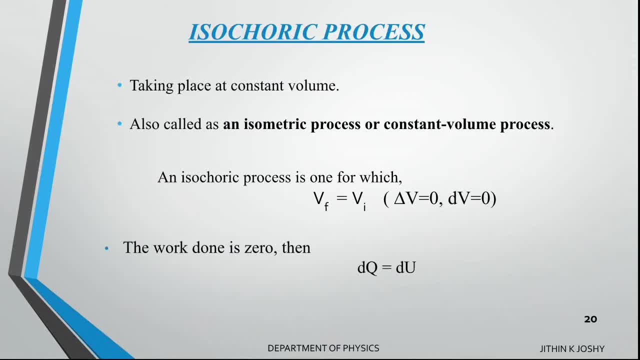 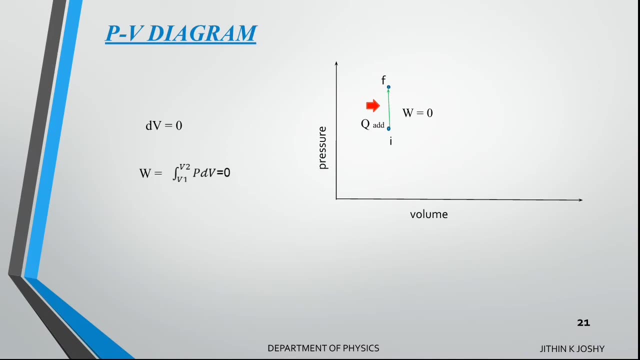 The work done in isochoric process is zero. So the change in the heat applied is equal to the change in internal energy, That is, dq is equal to du. Moving to the PV diagram, The two points marked, I and F, are the initial and final volumes. 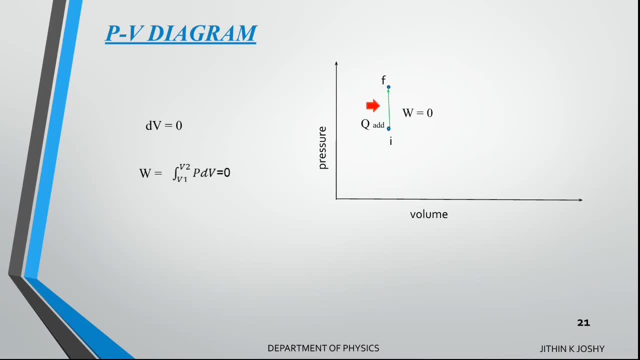 Since the volume is constant, We can say that Vf is equal to Vi, So dV is equal to zero. The work done is equal to PdV, Since we have two states, that is, the volume 1 and volume 2.. 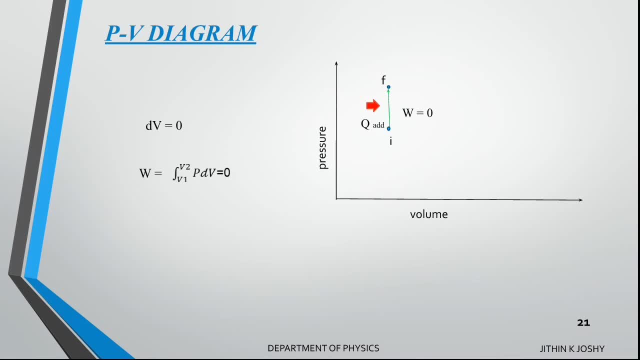 We had to use integration. So W is equal to integral, V1 to V2, PdV. We know that V1 is equal to V2.. So the change in volume dV is equal to zero. So the work becomes zero. In graphical explanation: 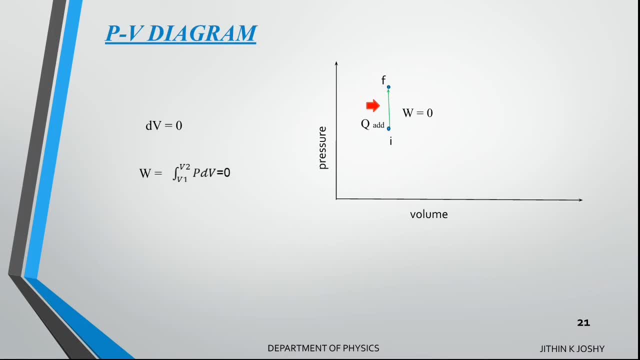 If we start from I to F, The volume remains constant, But the pressure P increases. Here the work done is zero. Why it is zero? From the PV diagram, The work done is the area under the curve, But this curve is purely vertical. 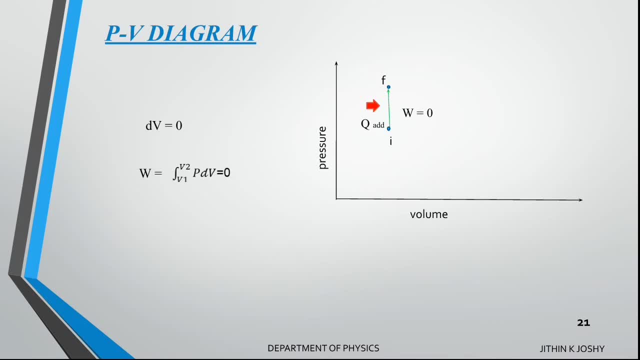 So no area, That is, the area is zero. It means the work is also zero. Using cold gas plus air mixture as fuel. Auto engine describes how the heat engine turns gasoline into motion. Like other thermodynamic cycles, This cycle turns chemical energy into thermal energy and then into motion. 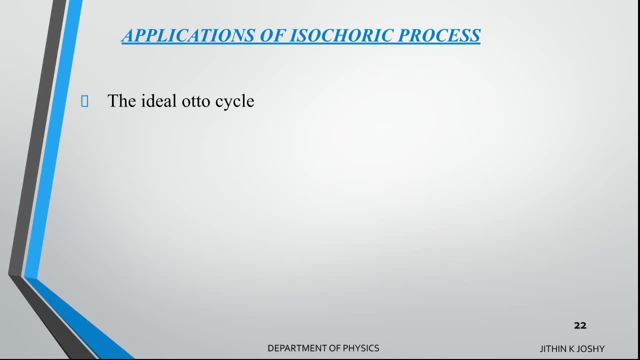 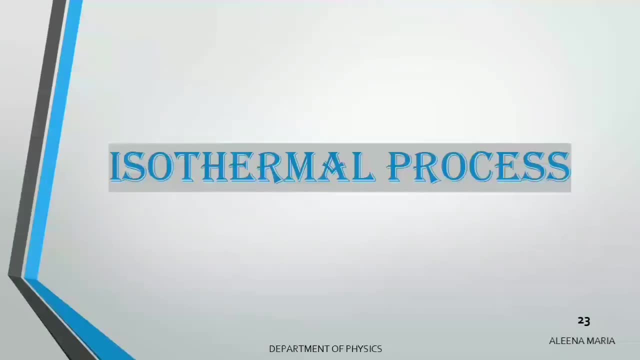 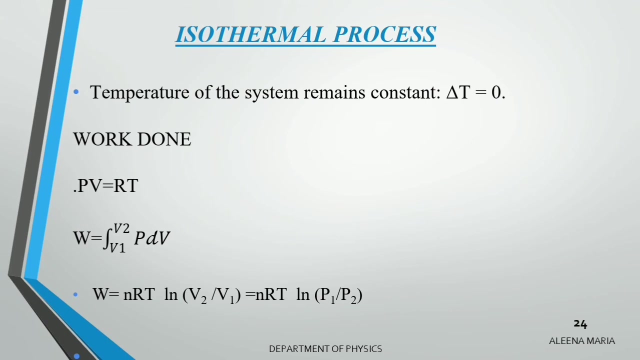 With this I conclude my part for the presentation on the topic isochoric process. Thank you. Now I am going to discuss about isothermal process, A very familiar but an important process. What is actually an isothermal process? It is a thermodynamic process that takes place at constant temperature. 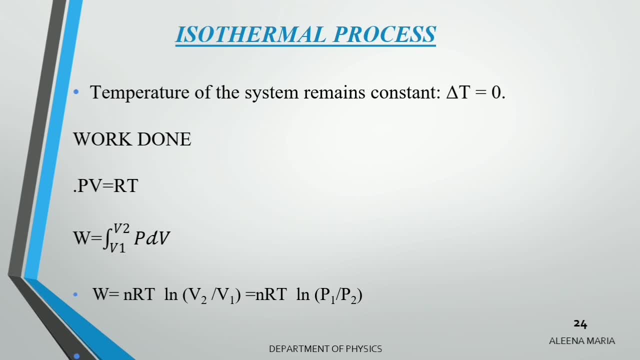 Whatever happens, Temperature remains constant. So in other words, We can say that There is no change in temperature, Or delta T is equal to zero. You can see a lot of examples regarding this isothermal process. The very best example is boiling of water. 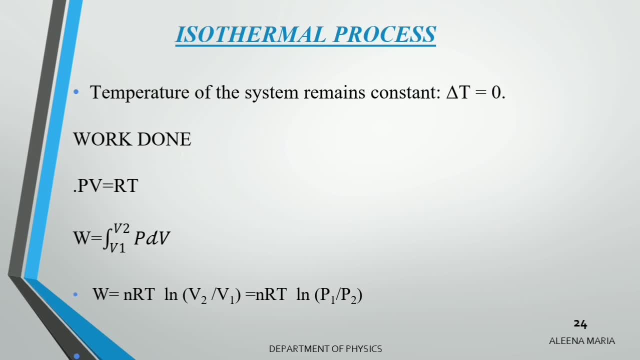 Whenever we boil water, We supply and heat, We supply and heat. It is actually an external supplier, So the heat supplied is used to break the bonds And to change the state from liquid to the vapor state, And there is no change in the temperature. 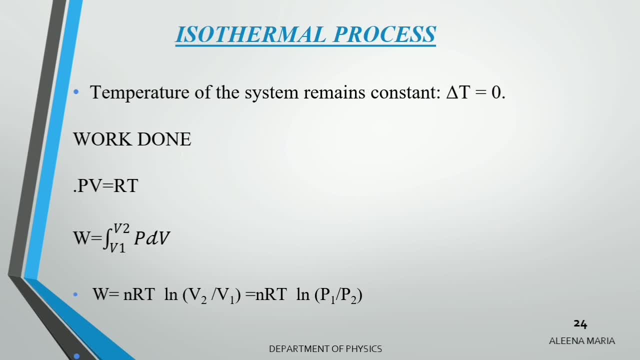 Now coming to the work done. We know the ideal gas equation is: PV is equal to RT And the work done equation is integral V1 to V2 PDV. So substituting for P From the ideal gas equation, We can write it as integral RT by VDV. 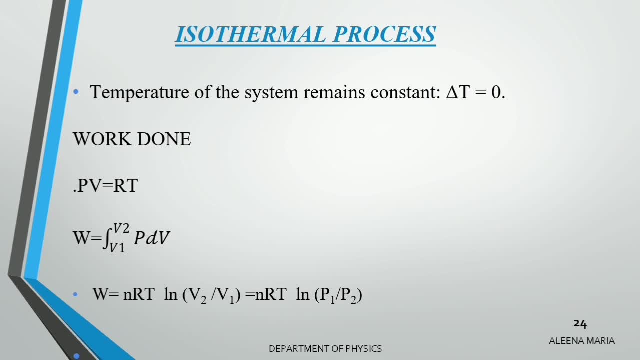 Integrating, We will be getting. W is equal to NRT log V2 by V1.. Or, in terms of pressure, We can write it as NRT log P1 by P2.. So this is how we find the work done for an isothermal process. 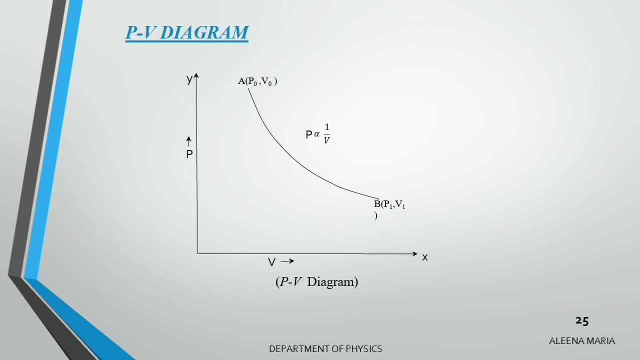 Now, coming to the PV diagram, We know PV is equal to RT. Temperature is equal to RT. Temperature is constant. Hence we can write: PV is equal to a constant, Or in other words, We can write it as: P is inversely proportional to V. 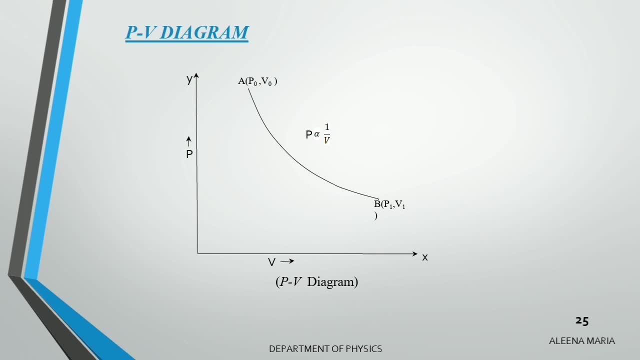 Hence, if we plot a graph, It looks like this: Here A and B are the two points, And A is the initial condition And B is the final condition, And we must note that Here the pressure and volume are the only that changes. 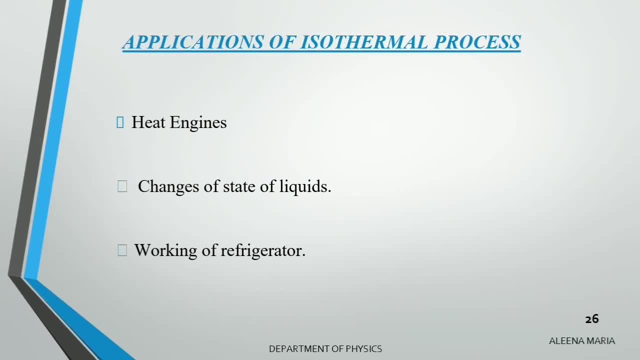 Now coming to the applications of isomers, Now coming to the applications of isothermal process. The first application is heat engine. Heat engine: they convert heat energy into mechanical energy. There is a source and a sink. Source is kept at high temperature, while sink is kept at lower temperature. 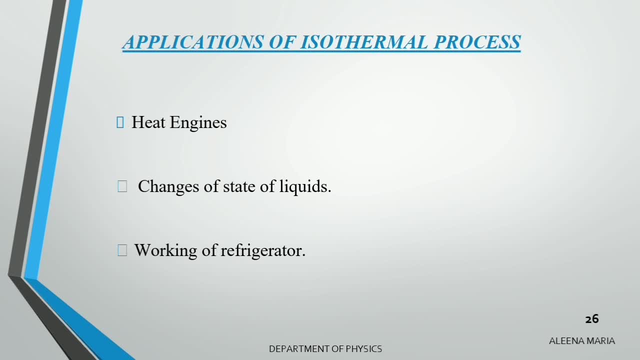 When the cylinder with the working substance placed on source, The pressure and volume of the gas changes, But the temperature doesn't change due to the infinite thermal capacity of the source. This is isothermal expansion. In the same way there is isothermal compression.